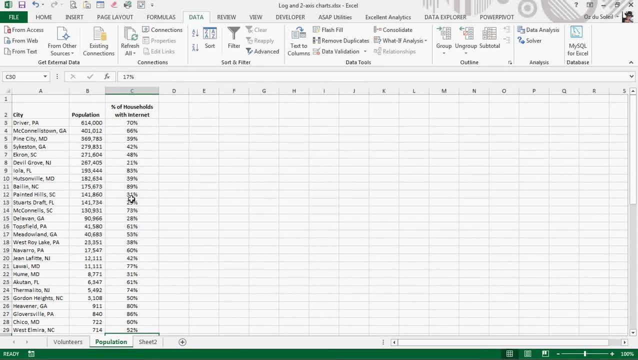 I'm going to look at population and the percent of households And I'm going to do with Internet. Let's click in my area and notice these are bogus cities and states. All right, These are all made up, So don't look at this as any type of accurate information. 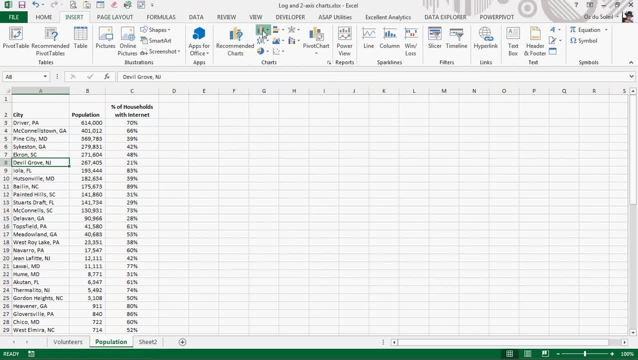 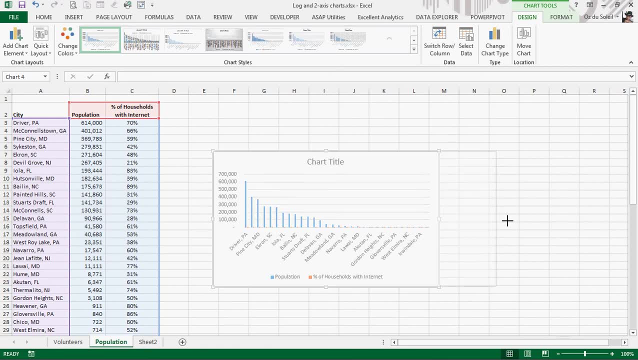 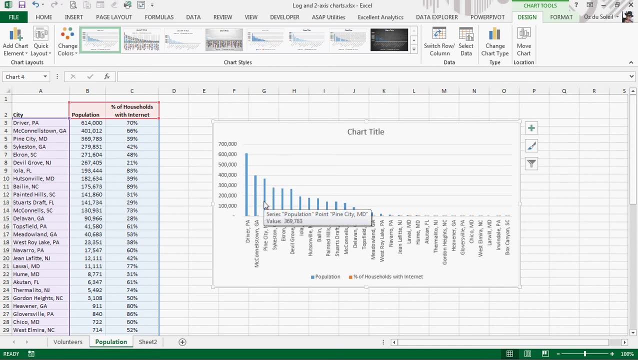 All right, Go insert Column graph. All right. Now what I want to do is turn this into a combo graph, All right. So I'm going to write because the percentages are really small, They're under one hundred thousand. These cities that are really small, they're under one hundred thousand and tiny. 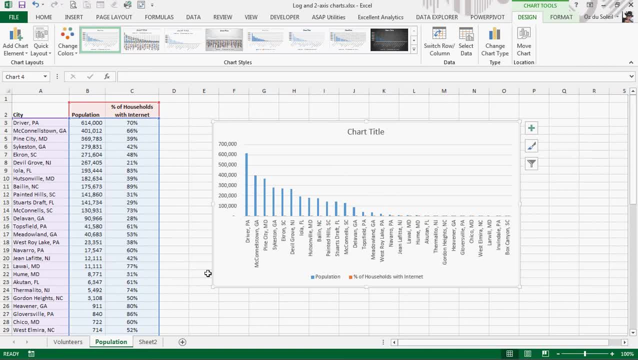 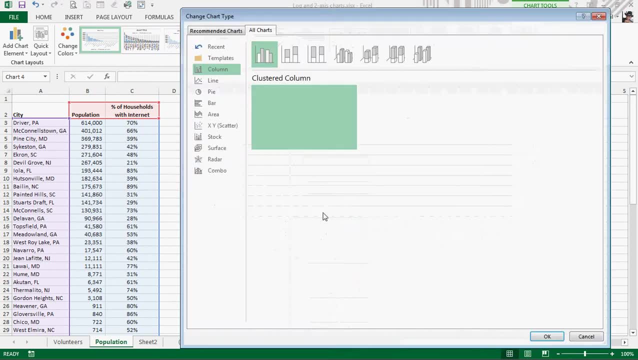 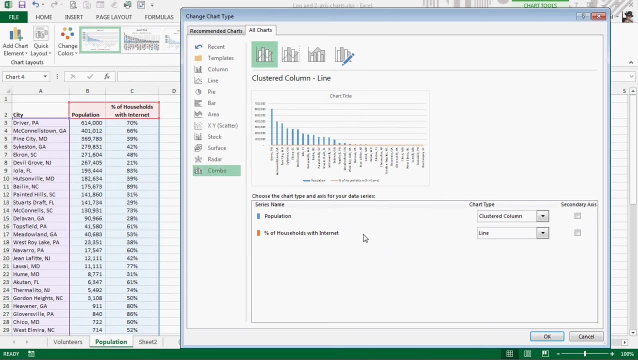 I can't see this. So nine hundred and eleven, I can't see that. So let's go ahead. Right click, Change chart type: Combo chart. And now I want to make Households with Internet a line graph, And I want it on a secondary axis. 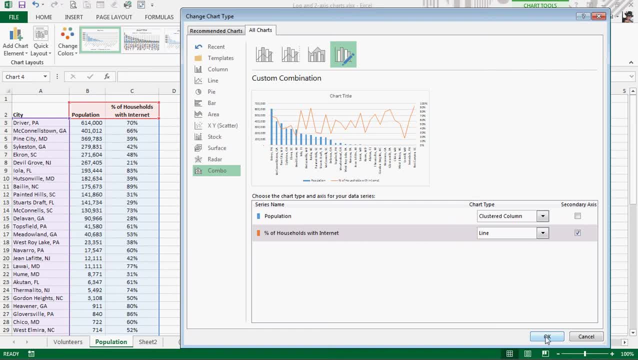 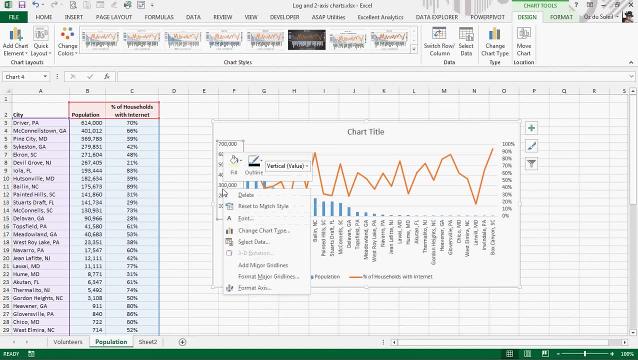 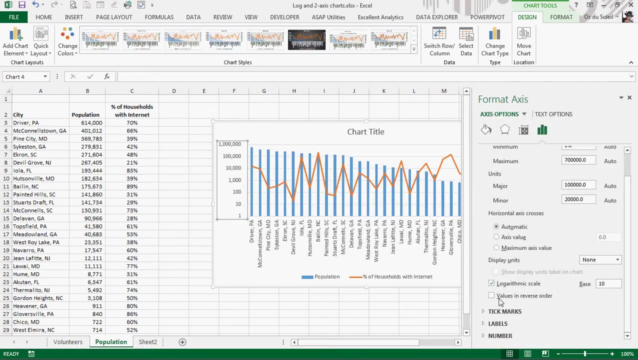 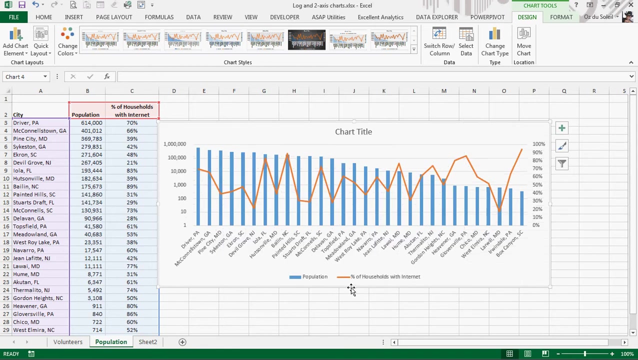 All right, You can see already the preview there. Great, Now let's take this and turn it into a logarithmic axis. All right, Now we can see. Now we can start doing some analysis and asking questions and looking at why is this? Topsfield, Pennsylvania. 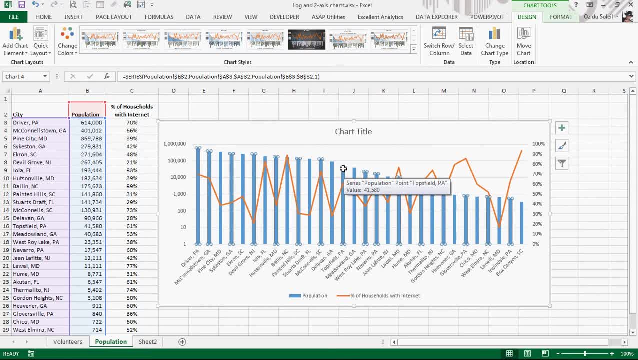 What's going on with its Forty one thousand five hundred and eighty people And it has sixty one percent Internet access And we've got ninety four percent of households In Box Canyon, South Carolina, have Internet And they only have three hundred fifty three people. Is there any kind of correlation? 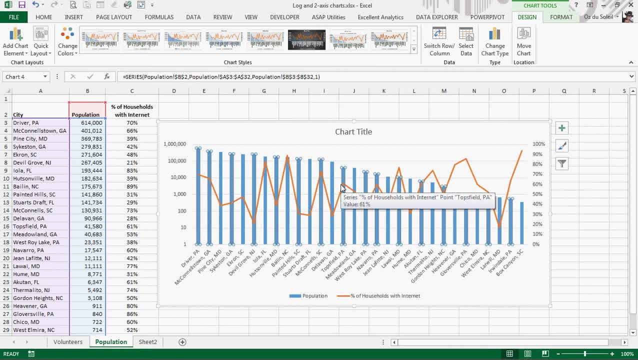 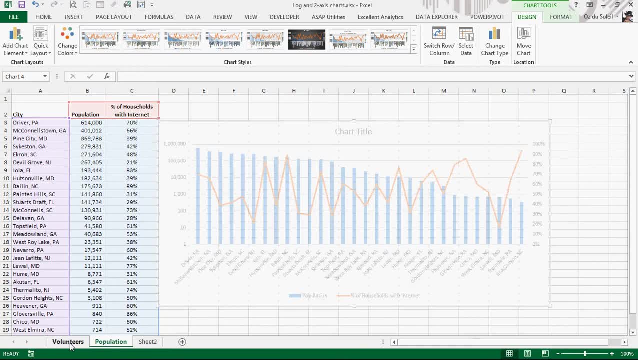 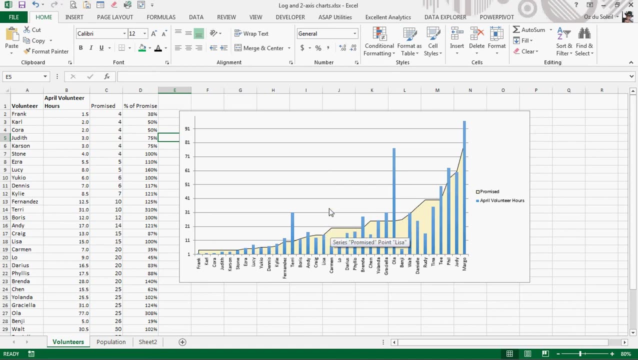 Well, go ask a real statistician, not me. I build the graphs, I don't do too much analysis, Right? Let's look at another example. Let's look at volunteers. So we're going to build this, All right. 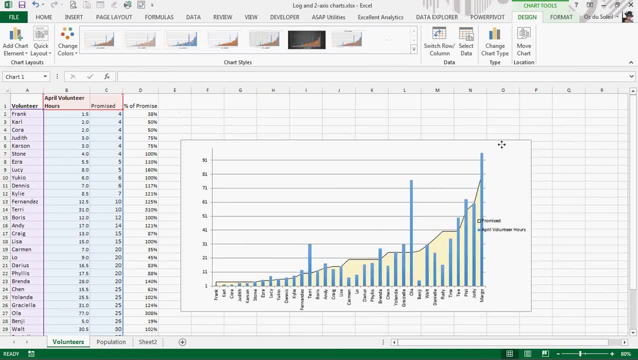 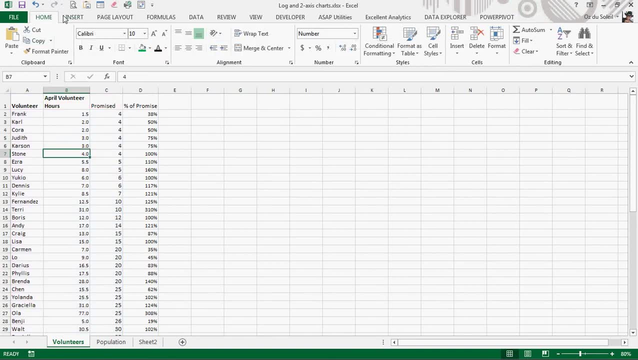 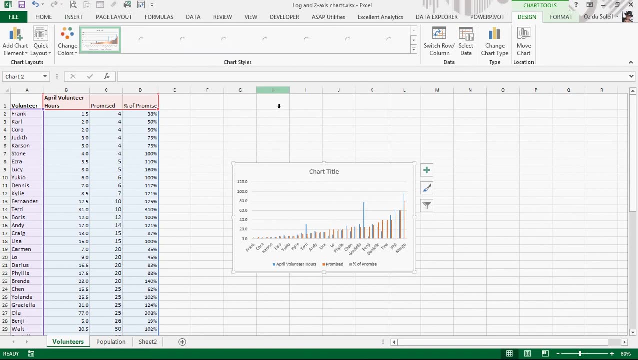 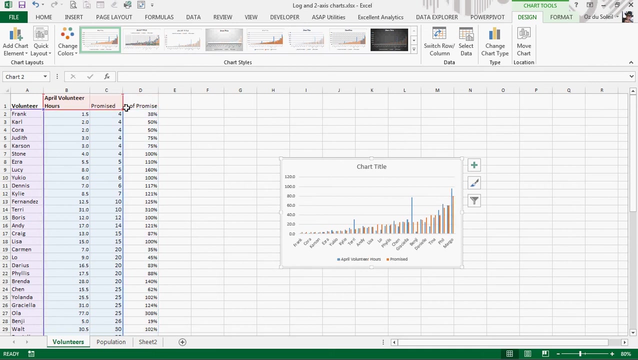 Get this out of the way. All right, Let's build this from scratch. Insert Column graph. OK, And I don't want the percent promised, So let's just slide this out of the way, All right. So now let's explain what we've got with this graph, or with this set of data. 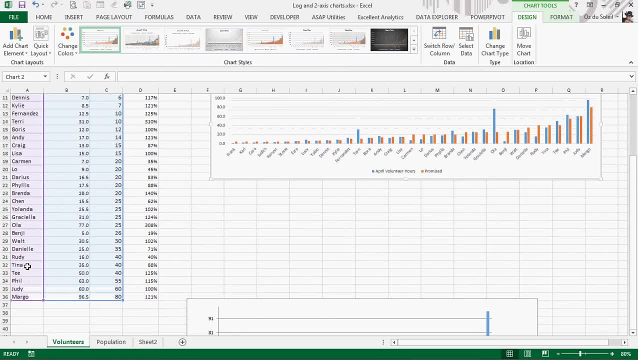 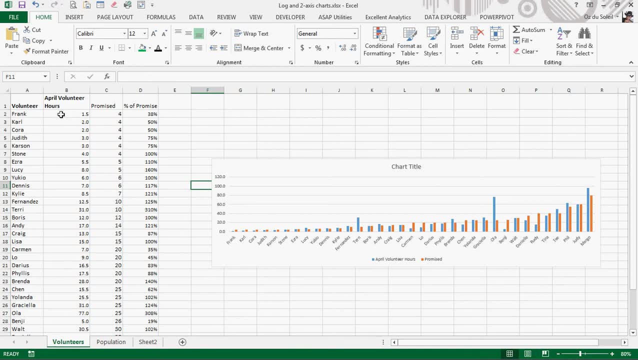 We have volunteers And the times that they promised that they would volunteer and the time that they actually volunteered in April. So we see that Yukio, promise six, delivered six. Lucy, promised five, delivered eight. Brenda, promised twenty, delivered twenty eight. Ola, twenty five, delivered seventy seven. 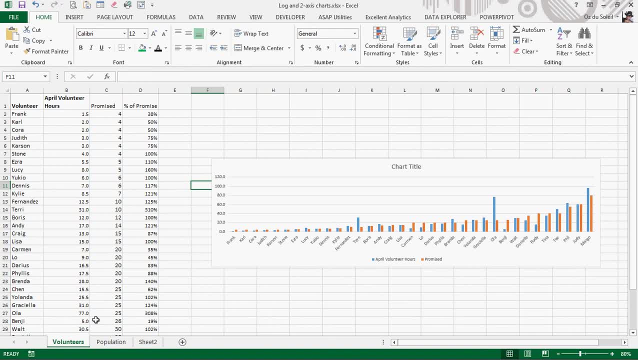 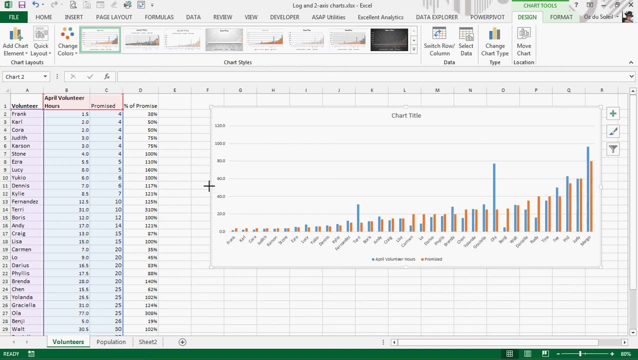 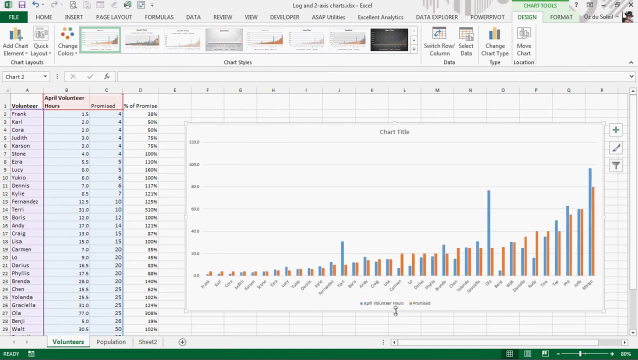 Oh, and Benji, promised twenty six, delivered five. OK, We might want to know these kind of things. Donors want to know. you know about volunteer hours, People that write checks for grants, And also just how are people doing with their promises? 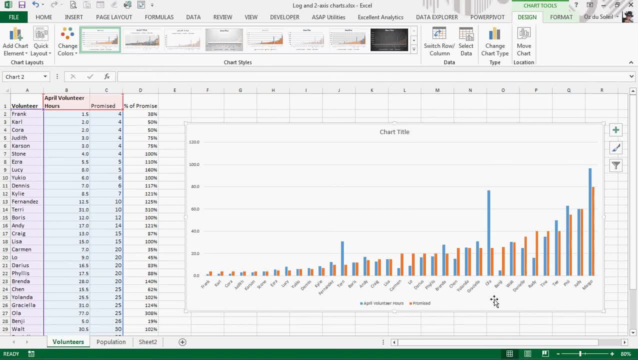 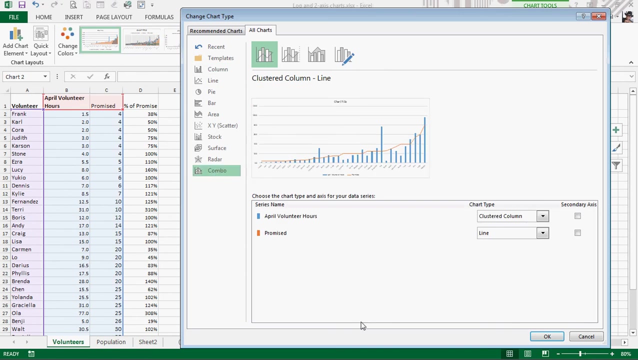 Are they just hanging out? Are they lying to us? What's going on? So, anyway, All right, Look at again. we have really small numbers and really big numbers. Let's go ahead and change this Change chart type. I want to change it to a combo graph and I'm going to leave everything on the primary axis, so I won't select anything for the secondary axis. 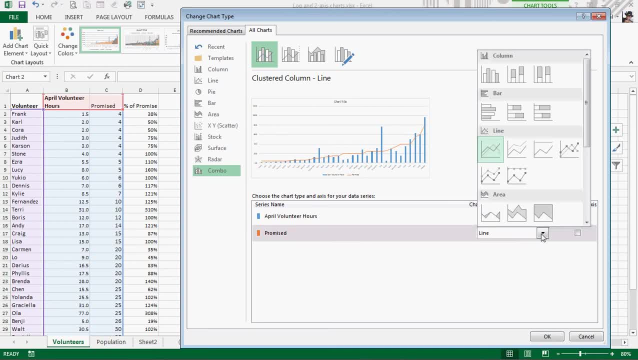 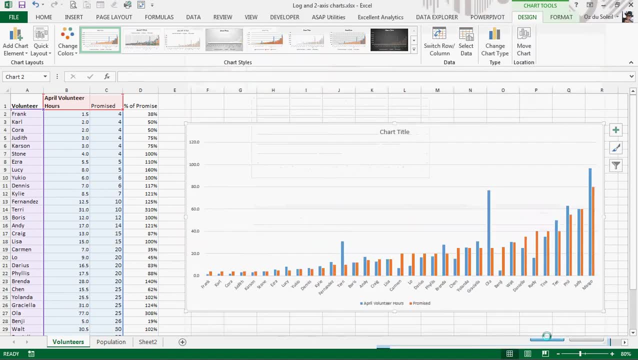 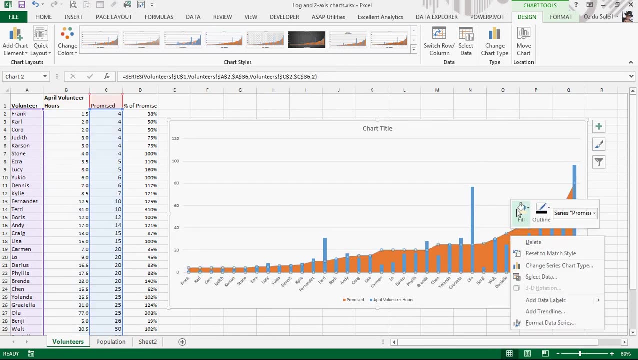 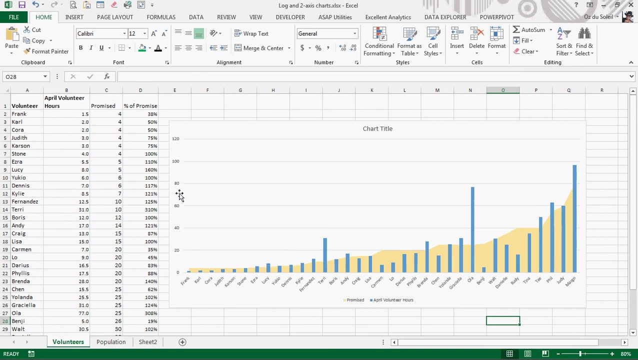 So promised. Let's make that an area graph. Good, OK, And that orange is a bit dark, So let's use Pale yellow works, All right. And in order to make sense of these really small numbers, let's go to the logarithmic axis.